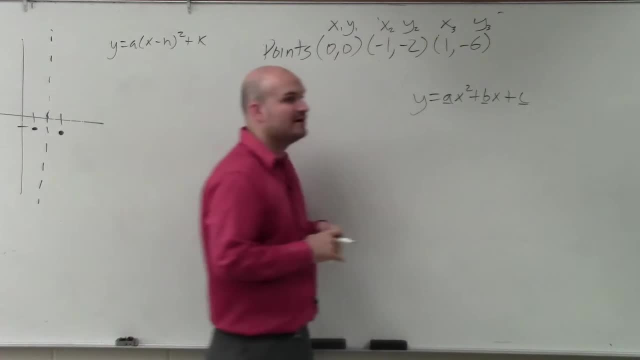 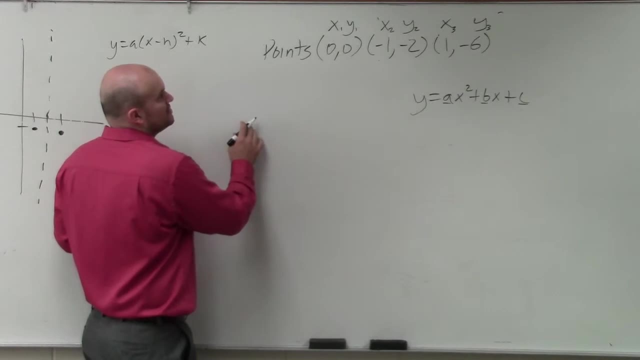 and you can see that here we have those three variables. So if we're creating three equations, we can solve for a, b and c, because we'll have three equations, which I'll show you here in just a second, So let's just go and plug them in. 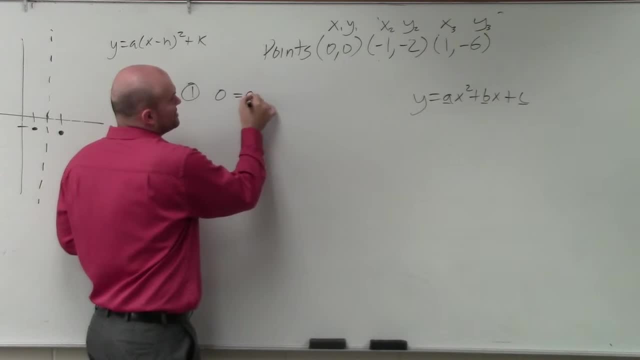 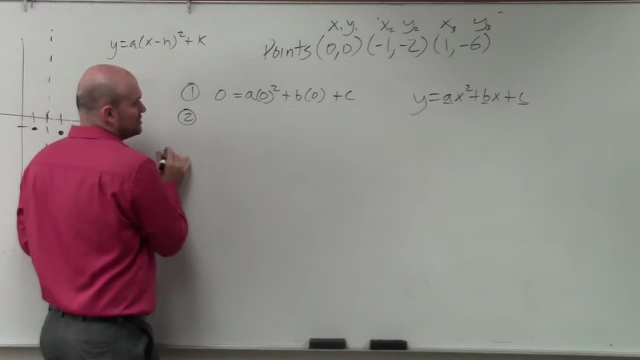 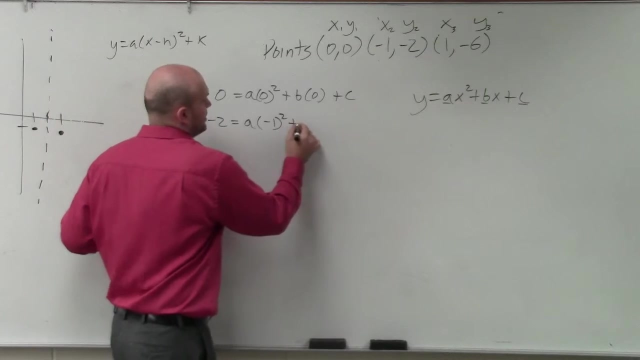 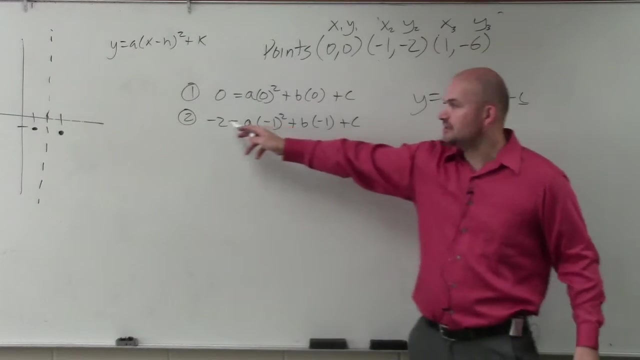 So we have: first equation would be: 0 equals a times 0 squared plus b times 0 plus c. Equation two is going to be negative: 2 equals a times times negative, 1 squared plus b times negative 1 plus c. All I'm doing is I'm plugging in x and y. 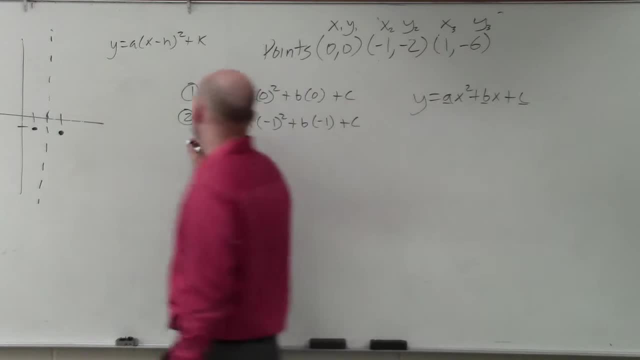 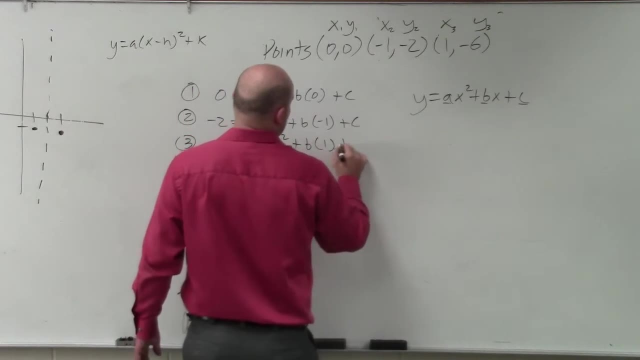 x and the y. Equation three is- I'm plugging in negative- 6 equals a times 1 squared plus b times 1 plus c. Does everybody see how I inputted the x values or the x coordinate for each graph into as the x? 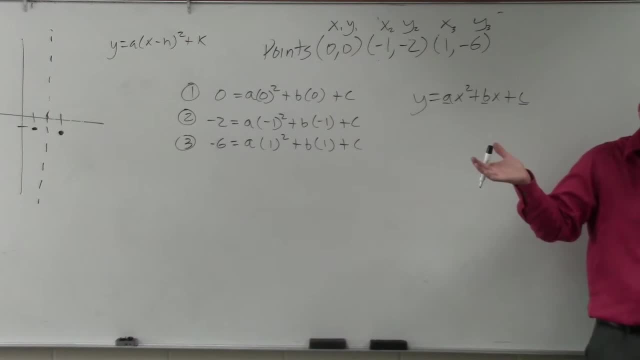 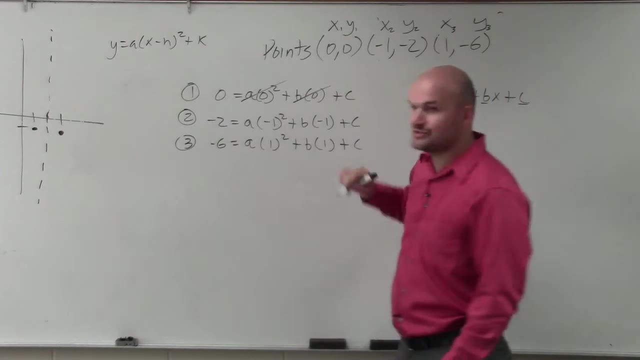 value for the equations. Does that make sense? And then I plugged in the y coordinates. Now we can go ahead and simplify this. Well, anything times 0,, ladies and gentlemen, is just going to be done. Could you move to a different seat please? 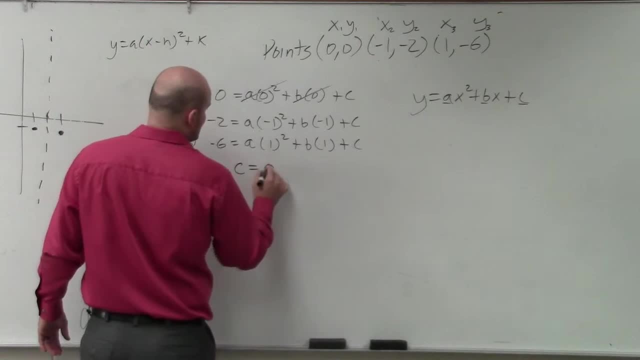 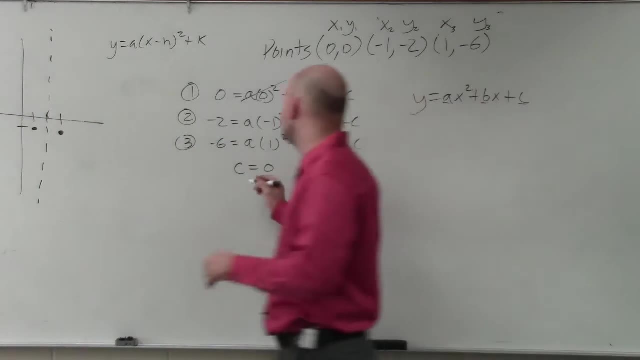 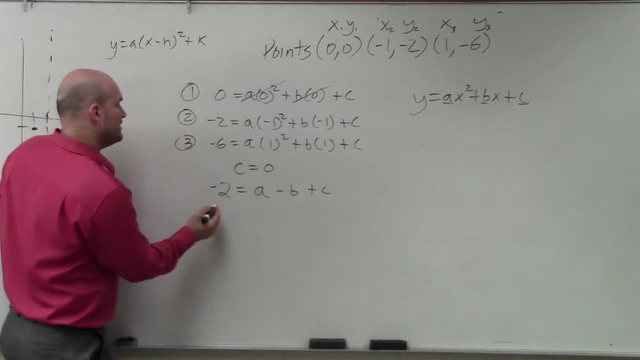 Thank you. So this turns out to be: c equals 0.. If we simplify this, we have negative 1, squared is 1. So that becomes negative. 2 equals a Minus b plus c. Then over here I have negative 6.. 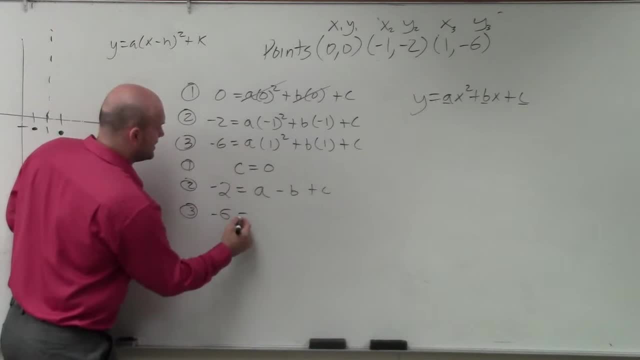 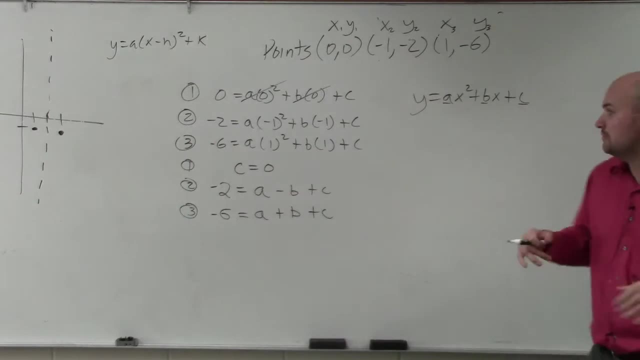 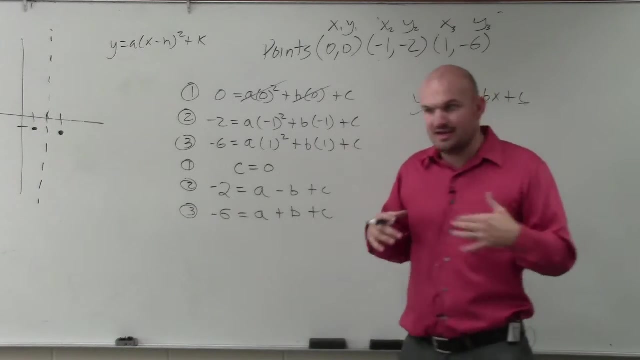 I'm just simplifying these equations. Negative 6, that becomes 1, equals a plus 1b plus c. Now we have three equations with three variables. We did not teach you guys how to solve a system of equations with three variables and three equations. 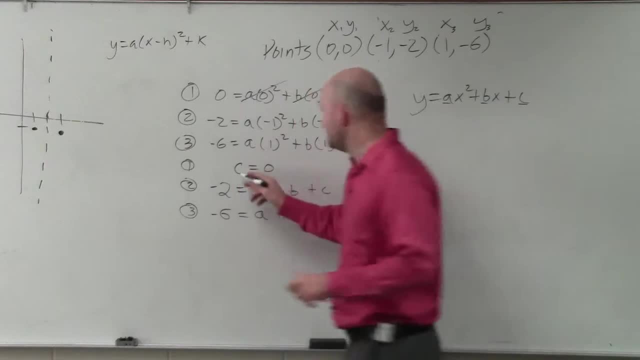 Fortunately though for you, we know when I simplify this equation. it tells us what the value of c is right, So I can just simply replace c with 0.. Well, am I adding 0?? Is that really doing anything? 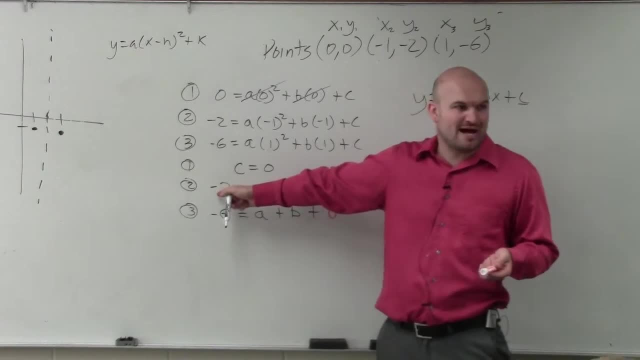 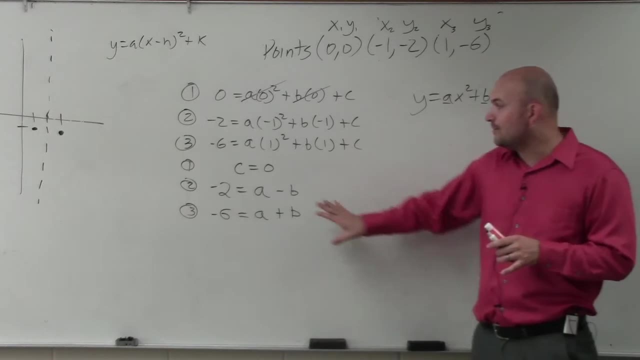 No, If that was like a number, you would have to subtract it or add it to get it to the other side, right? But in this case you basically have this. Now we already know what value c is. We need to solve for a and b. 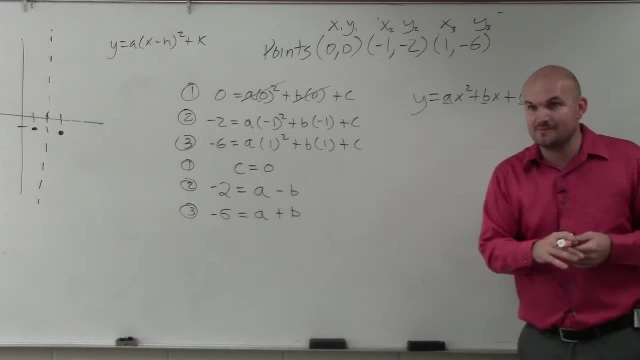 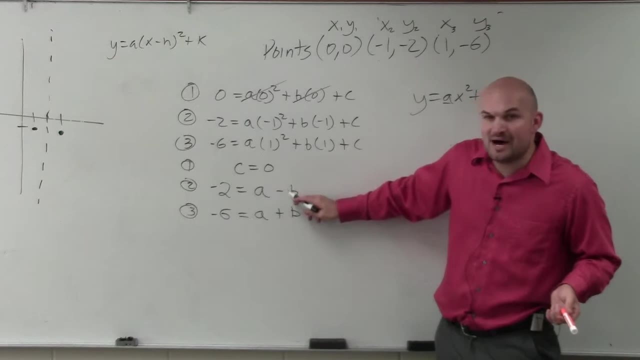 Does anybody remember what we would use? Yes, Elimination, You could use elimination, right, You could use substitution. but why use substitution when you have variables with a positive and negative and they have the same coefficients? So all I would simply do to solve this problem. 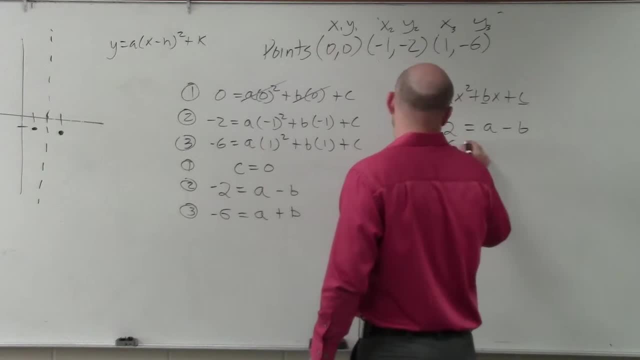 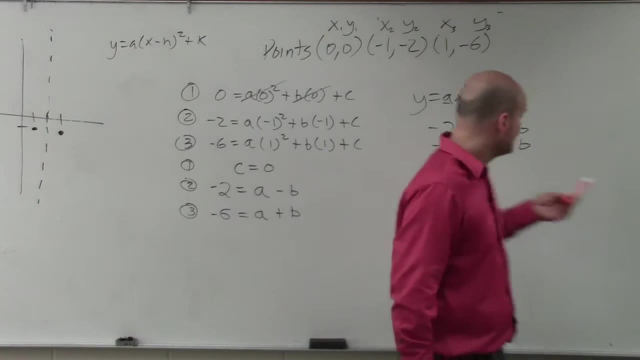 is, add negative 2 equals a minus b and add negative 6 equals a plus b. So make sure you guys go back and review systems of equations, elimination, substitution, because, as I mentioned, this was the easy one. This is a problem I could find. 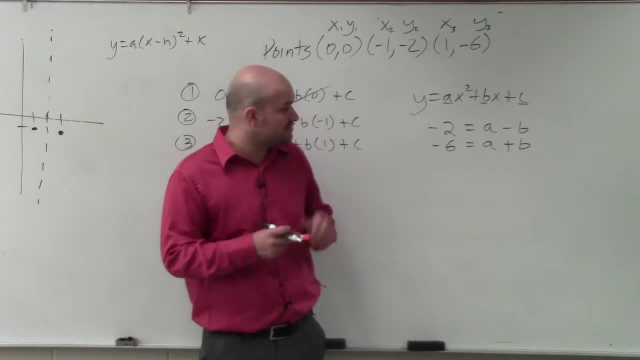 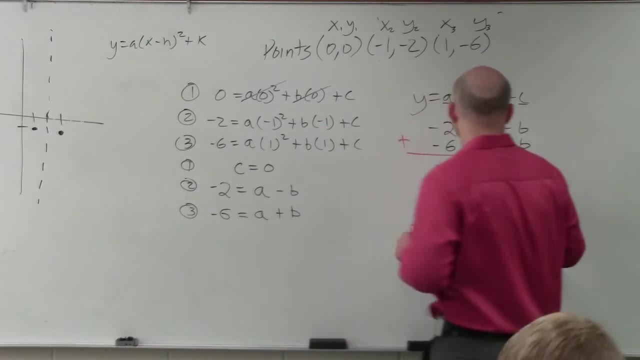 You might have harder ones, where you actually have to do some work for elimination, But in this case all I'd simply do is add the two equations. I get negative. 8 equals 2a. Those divide out, Divide by 2.. 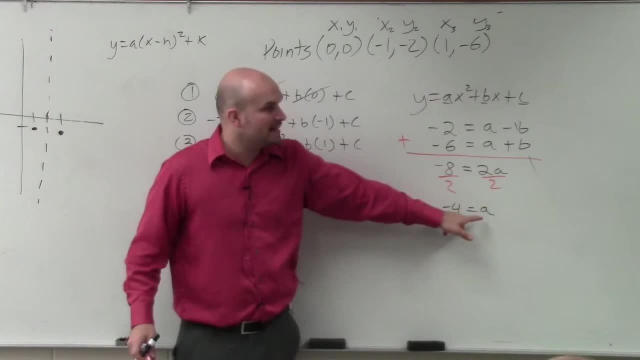 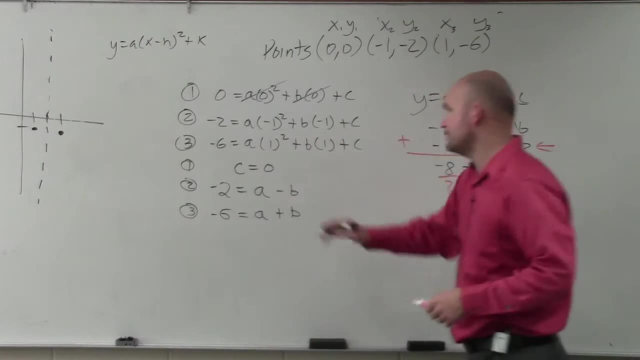 Negative 4 equals a. Then once I know what a is, I can plug it back into one of these equations to solve for b. I'll plug it into that equation or right over here. So I'd have negative 6 equals negative 4 plus b. 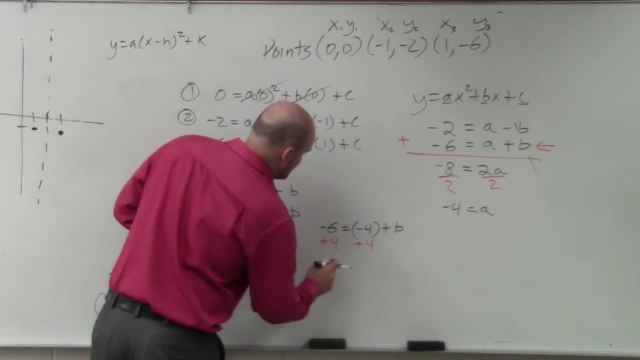 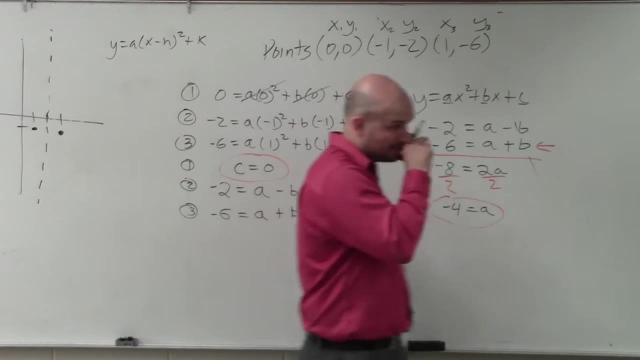 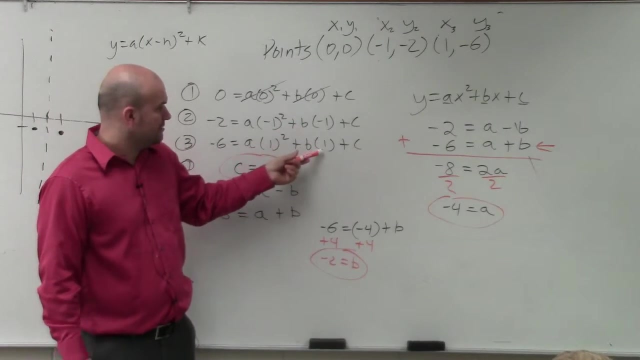 Add 4, add 4.. Negative 2 equals b. So I now know what b is, I now know what a is And I now know what c is. Yes, Where There This one. Just remember it's negative 1 squared. 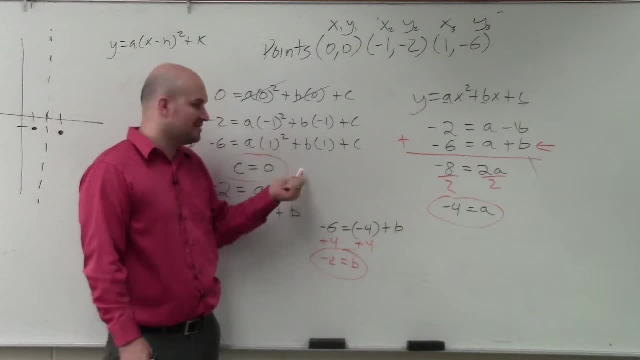 which means negative 1 times negative 1, which would be a positive 1.. Right, Negative times a negative would be a positive 1. It would be a positive. Yes, Does that matter in all equations? Nope, You could plug it into either one. 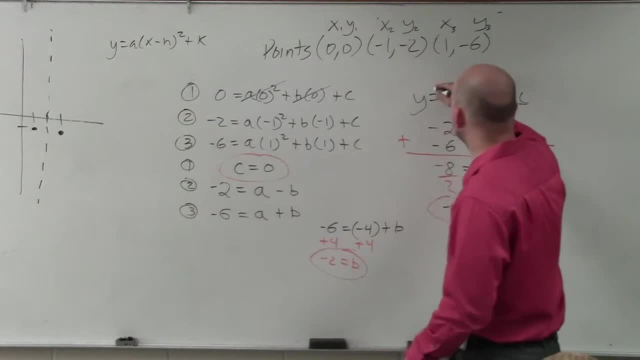 You would get the same answer. So now we know what a, b and c is. I'm just going to plug them in for this. So my final equation in standard form is: y equals negative 4x squared minus 2x and then plus 0,.